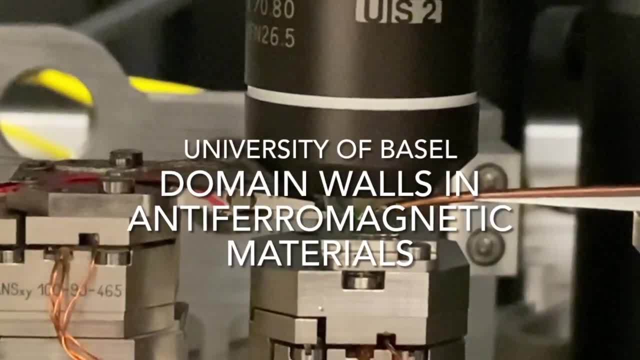 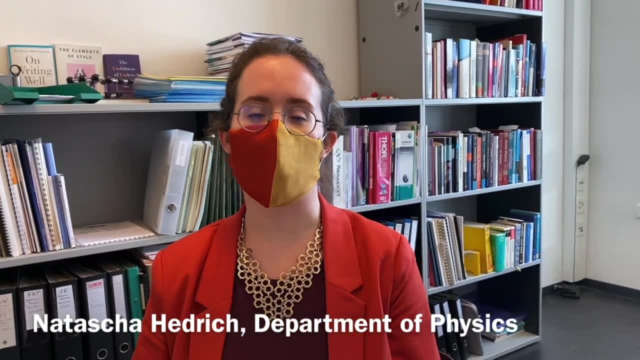 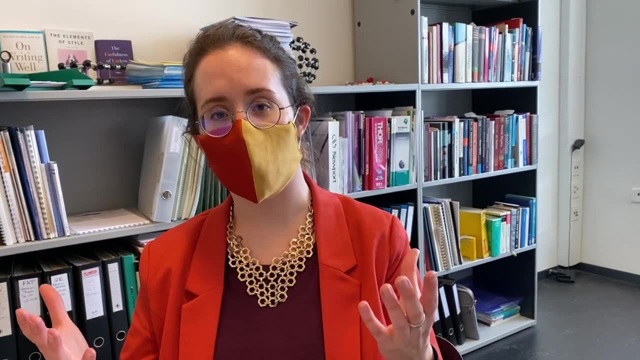 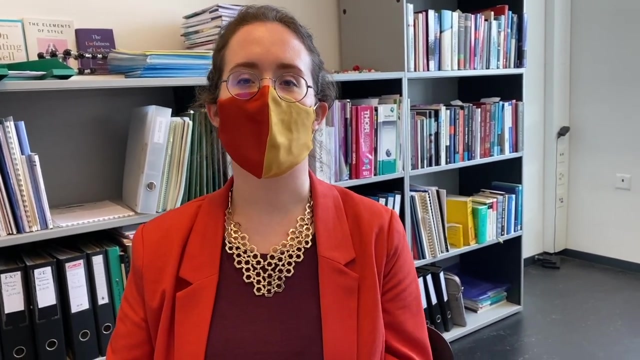 We were able to generate, measure and move domain walls in an anti-ferromagnetic system. What this means is you could use this as a potential for a memory device where you can move a domain wall. to define a bit which is either zero or one, To generate a domain wall. 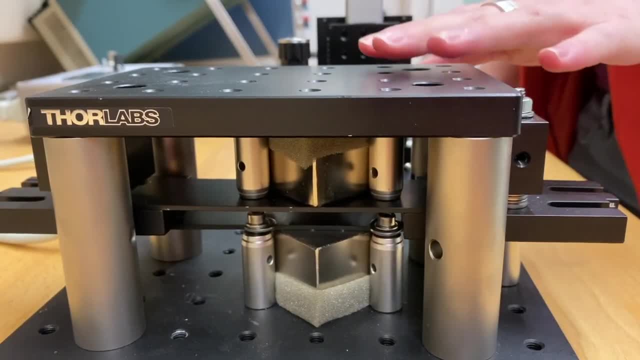 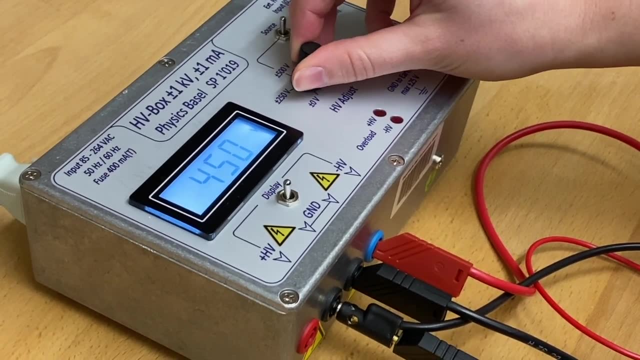 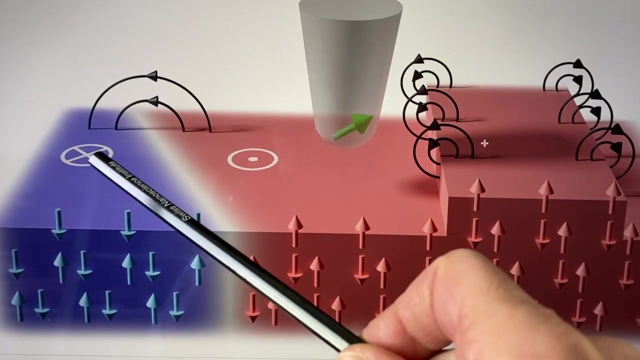 in an anti-ferromagnetic material we apply a magnetic and an electric field. By applying them parallel, we manage to create a certain orientation of the anti-ferromagnet. By applying them anti-parallel, you get the opposite orientation. Between these two you generate a domain wall. 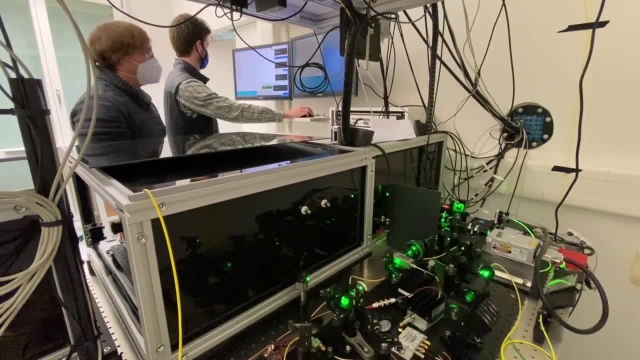 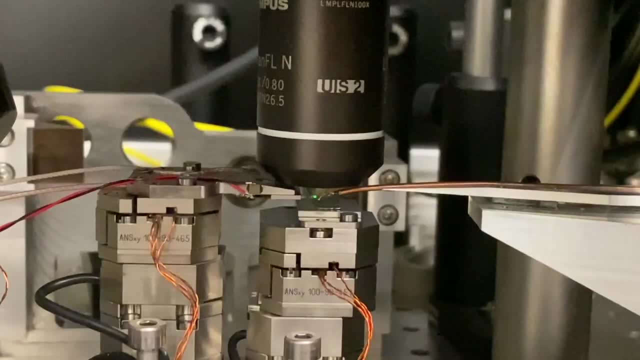 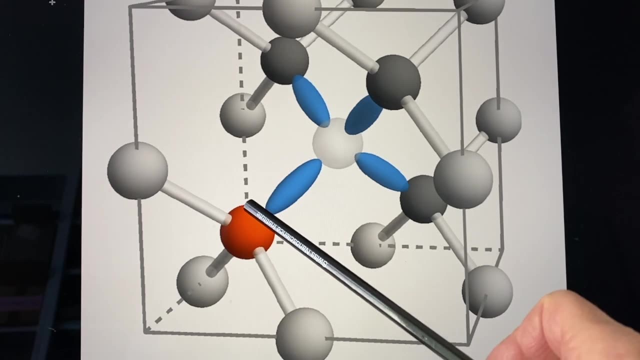 So, in order to measure the domain walls, we use a technology that's been developed in our group based on diamond defects, specifically one which is called the nitrogen vacancy or NV center. So here you have a nitrogen and a vacancy, and this creates a defect which is sensitive to magnetic fields. 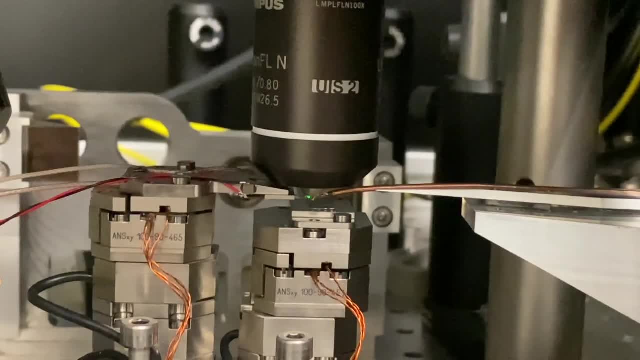 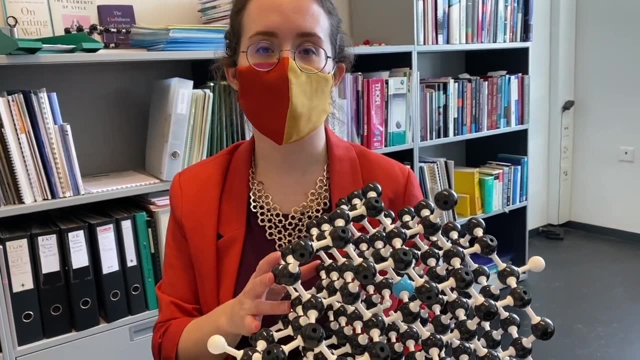 So by bringing this defect close to your anti-ferromagnetic surface, you can measure the stray magnetic fields that are produced, for example, from the domain wall. We found out that we can control where the domain walls are and we can measure the magnetic fields that are produced. 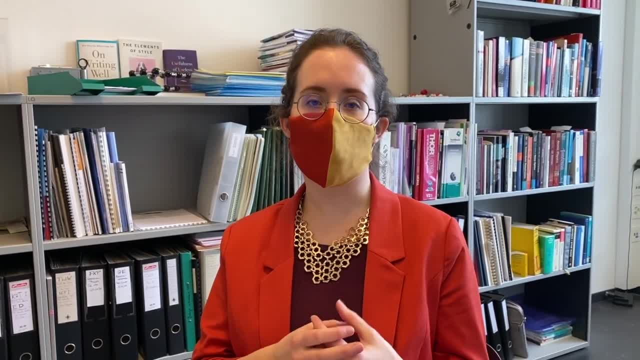 We can measure the magnetic fields that are produced by a laser, and we can also measure the denaturation of the domain wall, so we can measure the density at which the domain wall lies on the surface. And to do this we etch the surface such that what's left behind is just small square areas. 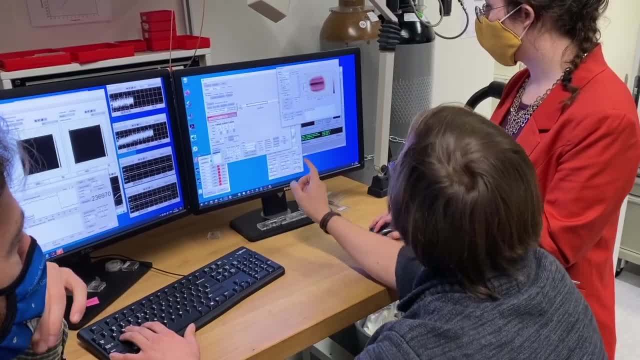 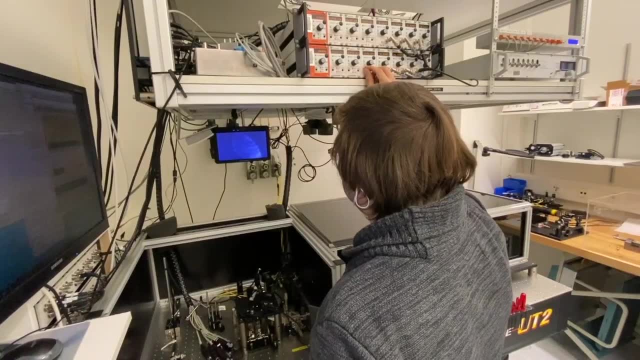 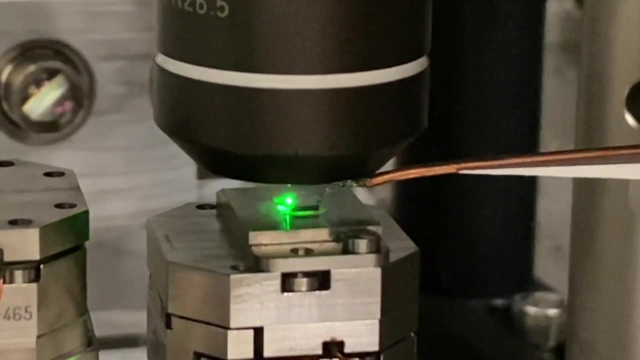 With this, the domain wall interacts with these squares and we can use the squares to direct where the domain wall goes. We also found that by heating the sample locally with a laser, you can move the domain wall repeatedly. And that's what we found is that the domain wall is actually more dense than the surface. 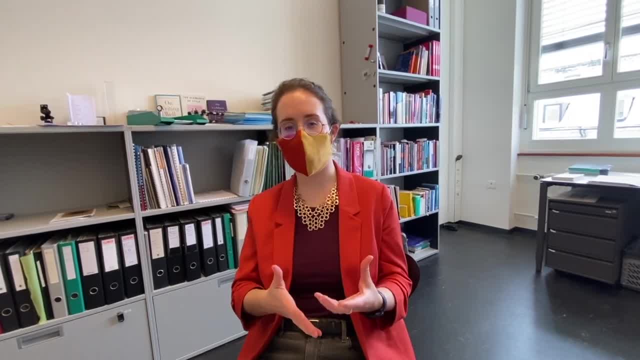 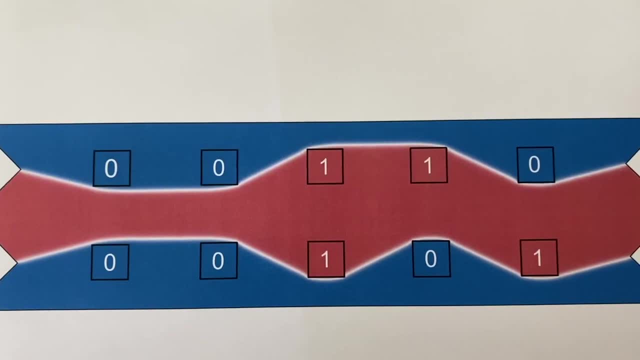 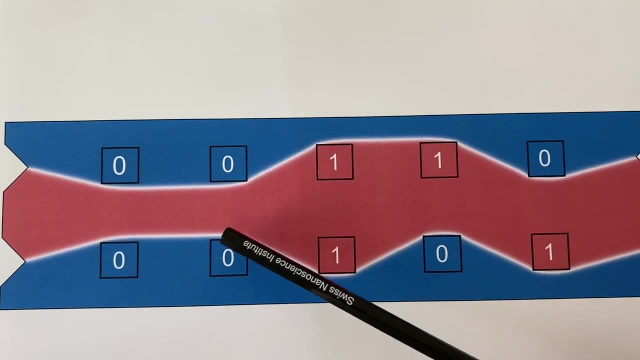 over these structures. Based on what we've been able to show, this gives us sort of a proof of concept of a type of antiferromagnetic memory. The small squares define the bit location and by moving the domain wall left or right from these squares, you can set the bit to either 0.